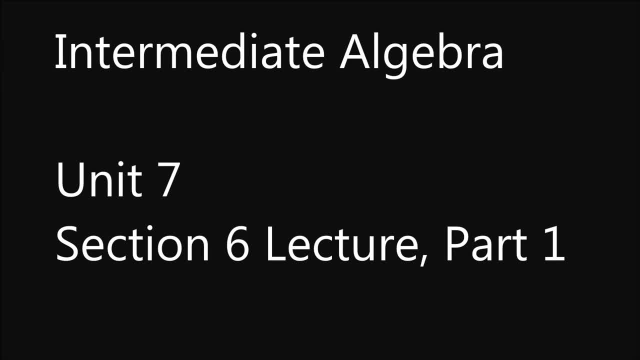 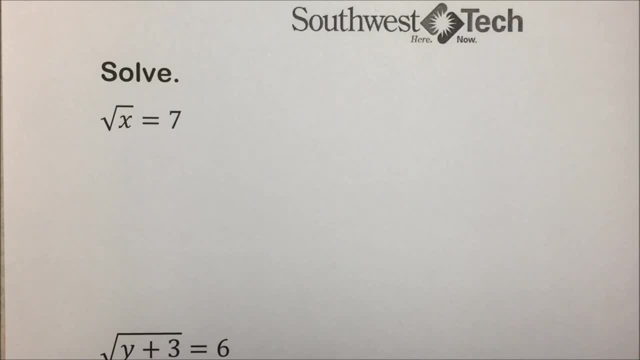 Section 7.6, Solving Radical Equations. To solve an equation with a radical term, we're going to isolate the radical term on one side of the equation and use the principle of powers and solve the resulting equation. The principle of powers is not always true, so we have to. 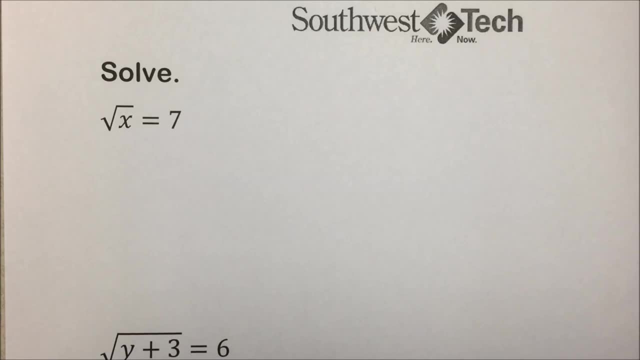 make certain that we check any possible solution in the original equation to see that it works. In this first example we have our radical isolated, so we're ready to use the principle of powers, which essentially says: whatever you raise, one side should equal in most cases. 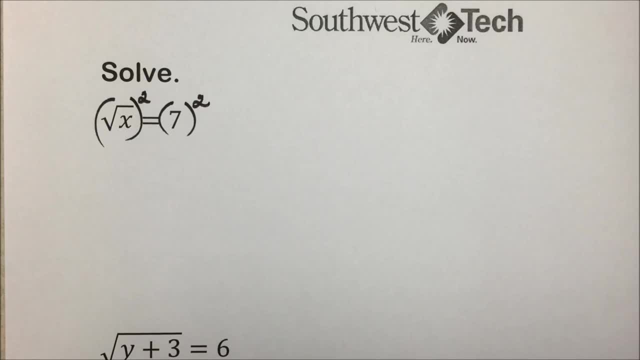 raising the other side of the equation to the same power. It's not always true. that's why we have to be sure that we're using the principle of powers. We check our solutions, But essentially this holds true and it's going to eliminate. 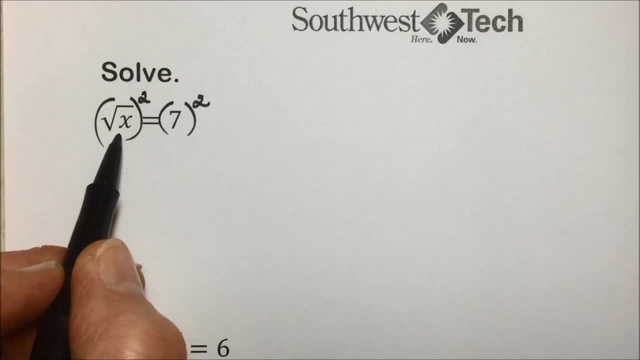 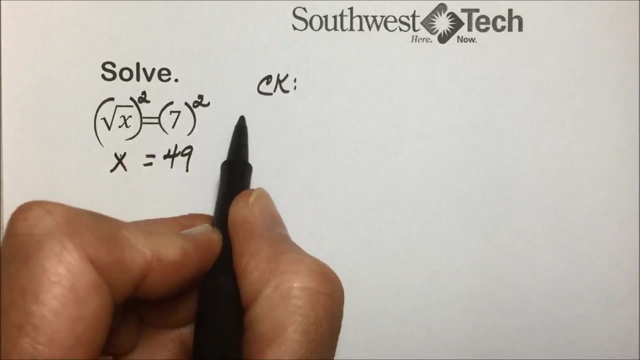 our radical Square root of x times square root of x is square root of x squared, which is essentially the radicand. 7 squared is 49.. There's nothing to do to solve, so we believe our solution is 49, and the check then would be to replace the variable with: 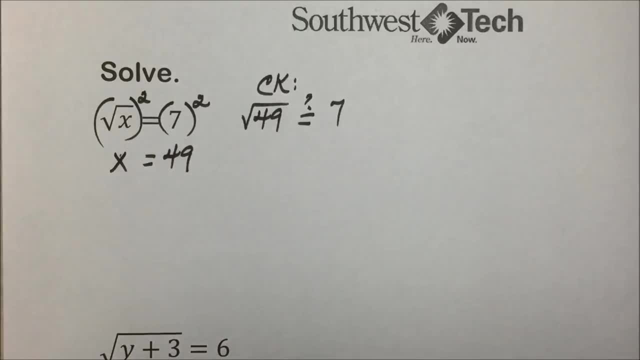 our value and see if we do get that expression. Recall, when we take the square root or have an even index. we always are looking for a non-negative solution, And so the square root of 49 is 7, and we have a true result. so 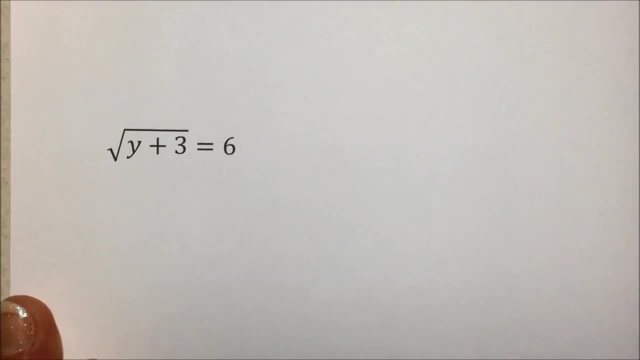 our solution to this problem is 49.. In this next problem, our first step always is to isolate the radical. that's already done for us. To undo a square root, we will square it one side we do to the other, using the principle of powers, Squaring a square root or a radical. 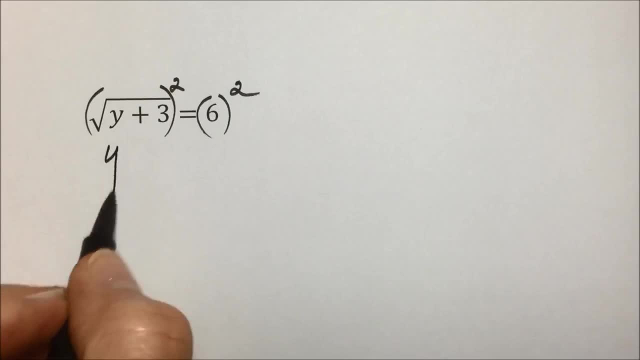 with an indice of 2 means we are going to get our radicand. on the right hand side, 36 is the result of 6 squared, and the only thing left to do to get y or our variable by itself is to subtract a 3 from each side and we end up with y is equal to 33.. Before we are done, 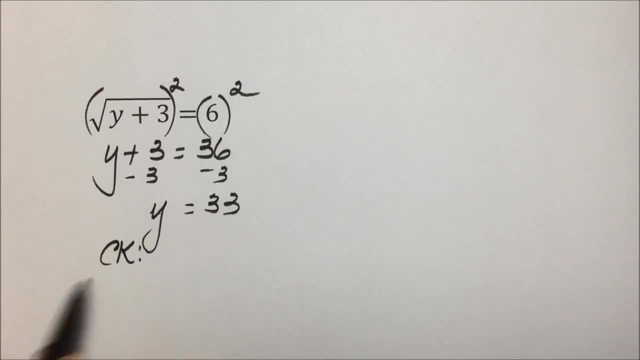 with the problem, though we want to make sure that that does work, because of the possibility that the principle of powers is not always true and sometimes it generates what we call an extraneous root, a solution that doesn't work, But let's see if it works here. Replacing 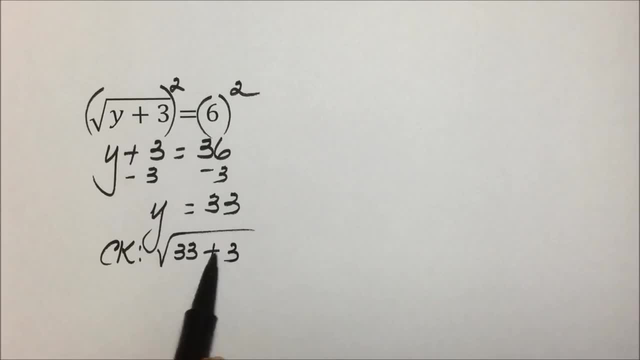 y with 33 plus 3 into the original equation. we'll see if it does in fact give us a result of 6.. Well, 33 plus 3 is 36, and the square root of 36 is 6.. So we can accept our solution. 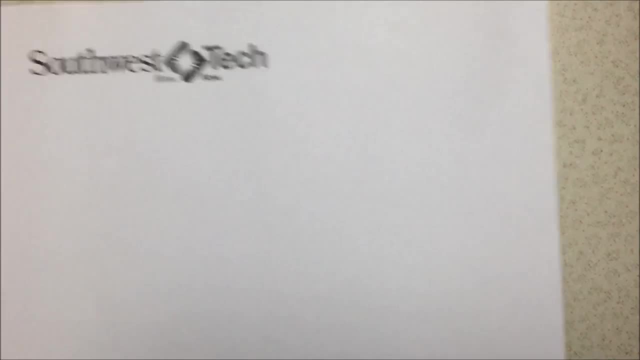 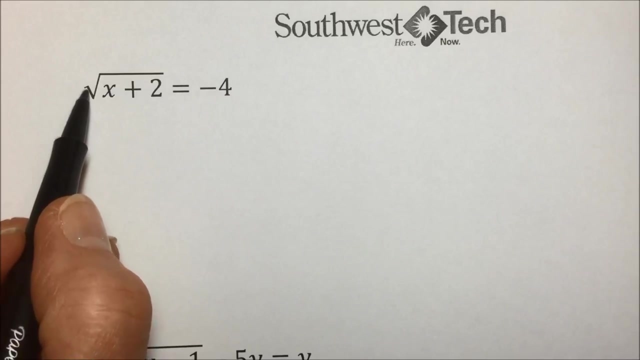 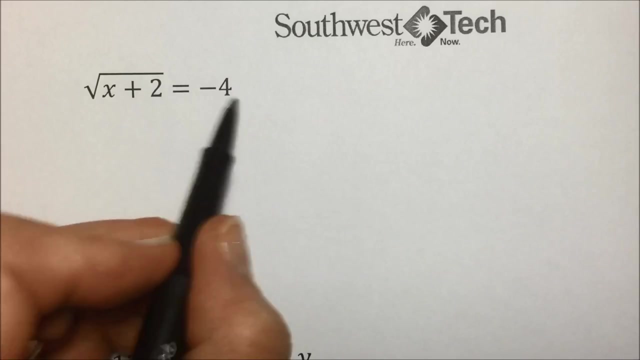 for that particular problem. In this next example they're asking us to solve this radical equation And right off the bat, we have a problem. When you take the square root or an even indice, we always are looking for a non-negative solution and they are asking us: could this? 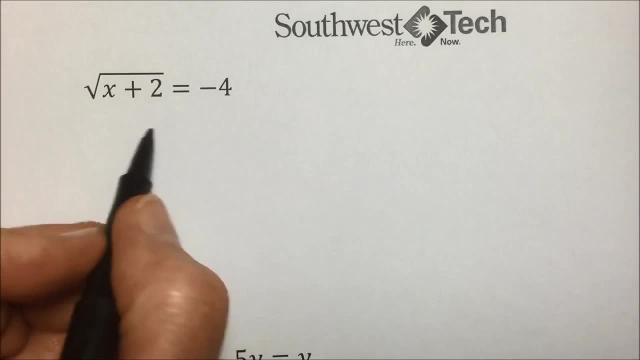 be equal a negative 4. Because it's a negative, there is no solution that would be possible to the square root had it been a cube or a fifth, some odd Comic, because every square root is an even indice in f, so the right hand side problem does always apply here. future. 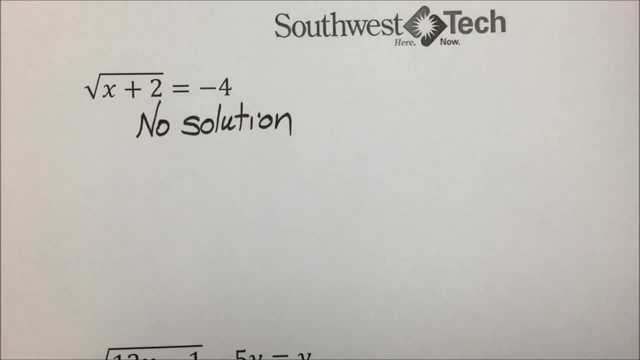 above, that would be uglyiają. A is the area below x1. in fact, we have again no solution for this form of number. needing a fifth, some odd indices, we would be able to do something and come up with a possible solution. 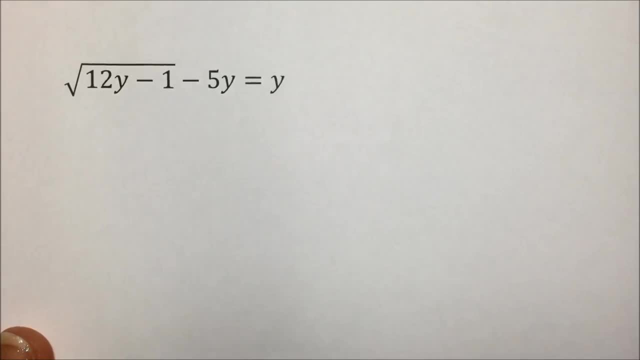 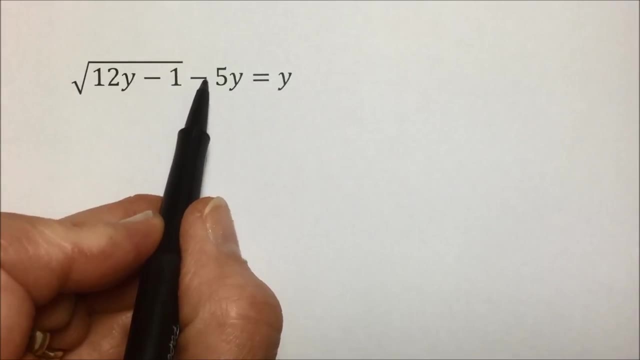 In this next radical equation, we do need to make sure that our radical is by itself. The radical has a subtraction of 5y and if we squared both sides we would end up having a binomial here, and if we can avoid that, that's what we're going to do and that's why it's. 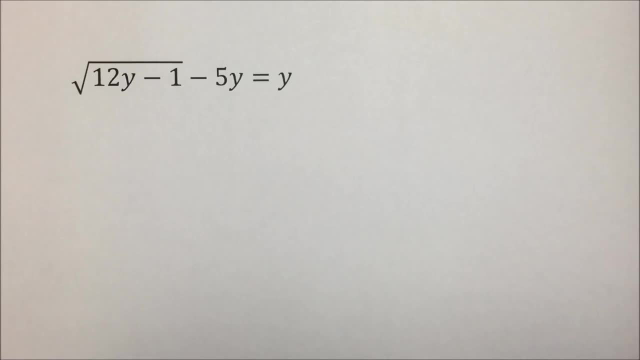 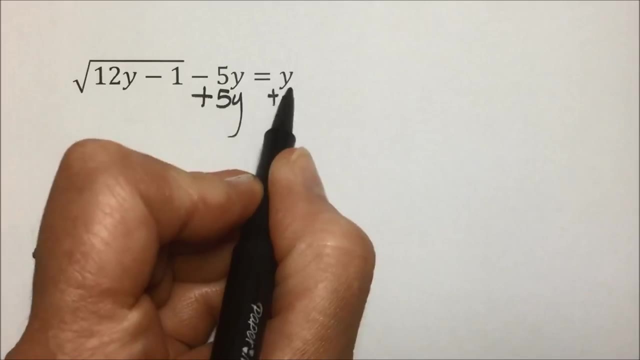 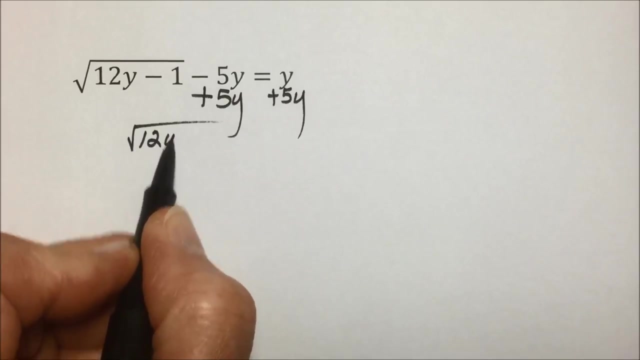 important to isolate your radical term on one side of the equation before you use the principle of powers. So, having said that, I'm going to add a 5y to both sides to get the radical by itself. We now have the square root of 12y minus 1 on the left and 1y plus. 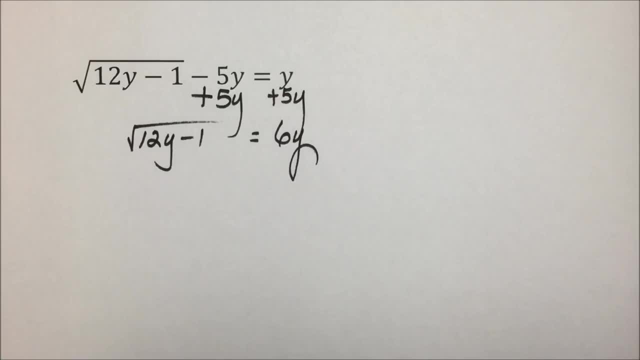 5y is 6y. Step 1 is done. as far as isolating the radical, We're now ready to undo the square root by squaring. Using the principle of powers, we square both sides Square root of 12y minus 1 times square. 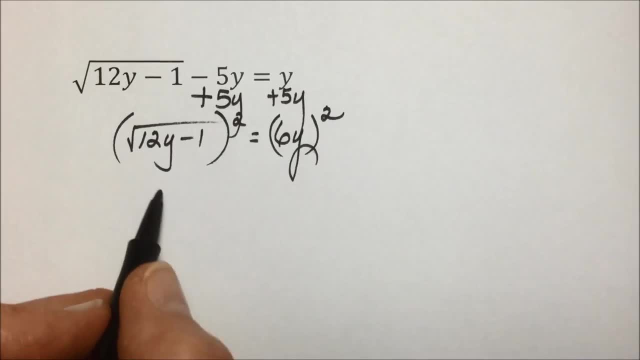 root of 12y minus 1 gives us two of those and the square root of a pair is that factor of 12 minus y. the radicand 6y squared is 36y squared. We have different degrees on our variables. This looks like the main variable is going to be 6y squared, The second variable 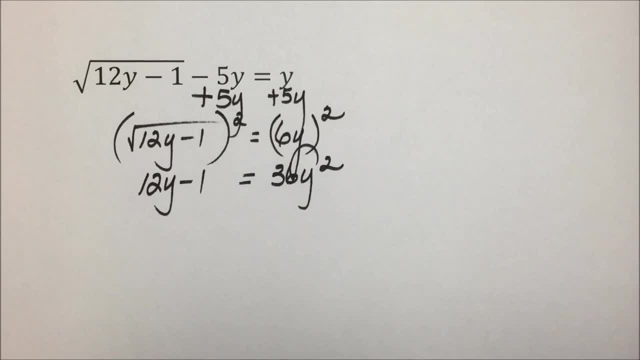 makings of a quadratic equation that we are going to have to factor and use our zero product property. So I'm moving everything to the right, which changes its sign when we take a term to the other side. Positive 12y taken to the right becomes a negative 12y. Negative: 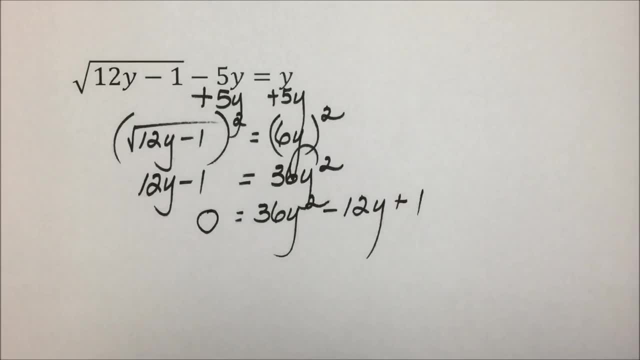 1 taken to the right, becomes a positive 1.. And you can see that if you subtracted a 12y from both sides and added a 1 to both sides, we would have this result. Is it factorable? We recognize the first term is a perfect square. It's 6y. The last term is a perfect square. 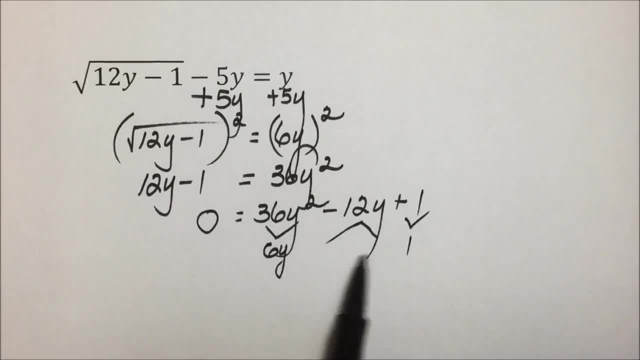 And for this to be a perfect trinomial square, we multiply the square root of the first and the last term and double it and see if that is the middle term, And it is. So this ends up factoring into 6y with a 1.. 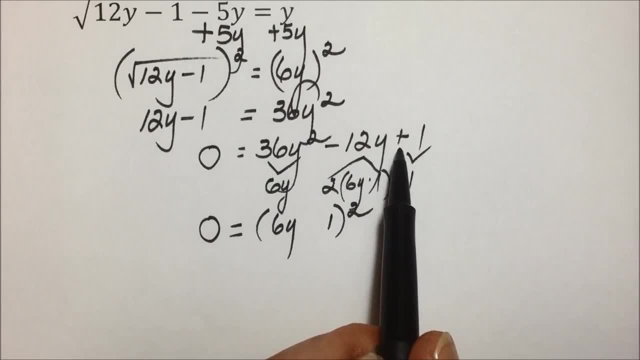 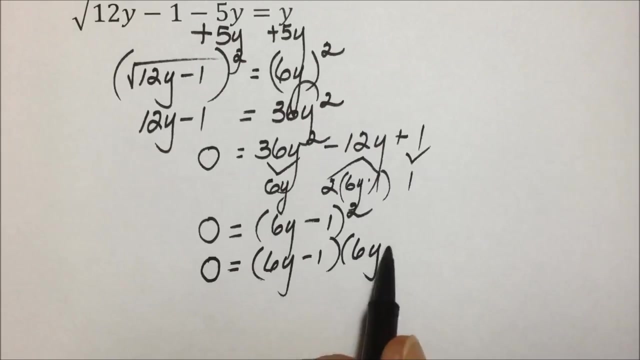 Quantity squared. Both signs in our binomial are the same. Both are a minus. Solving this: we're looking for terms that equal zero And since both of these factors are the same, and to help you see that this is equivalent to 6y minus 1 times 6y minus 1. We have two. 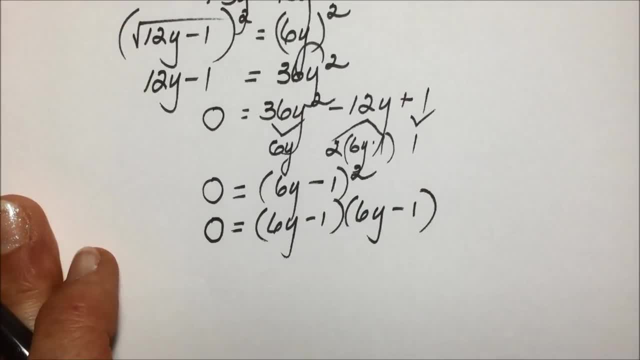 things multiplied to give us zero By the zero property. it says that either 6y minus 1 equals zero or 6y minus 1 equals zero. We have a redundancy here, so we only need to set one of these factors equal to. 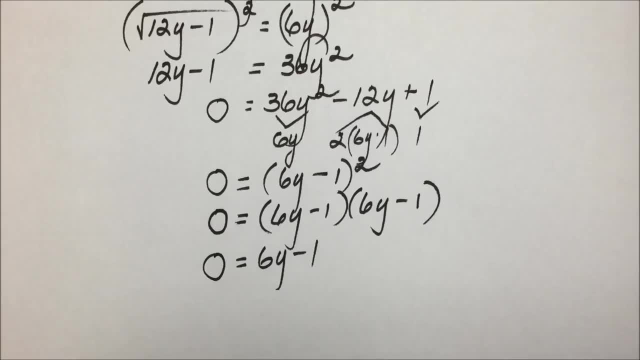 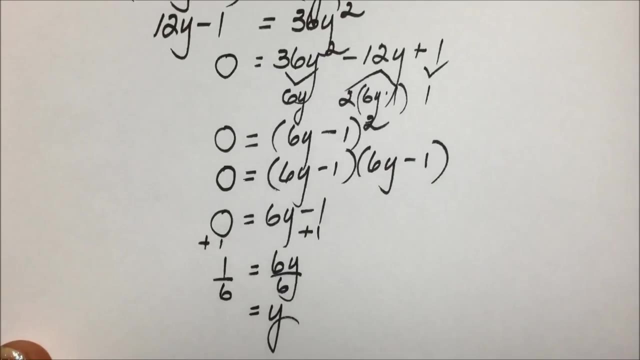 zero and solve to find the value that does result in a zero. So adding a 1 to both sides or taking that 1 to the other side gives us the following: And dividing both sides by six to get zero, Y times the kingdom of y was equal to zero. The problem is solved with the solution of. 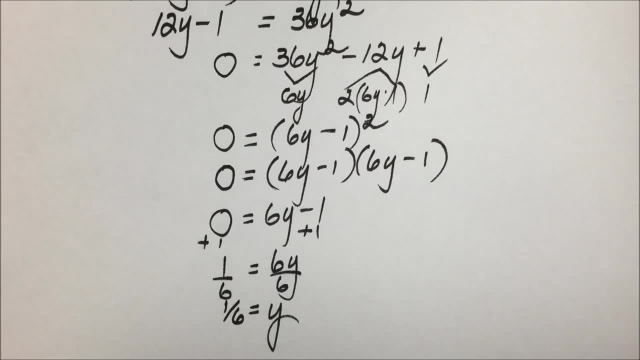 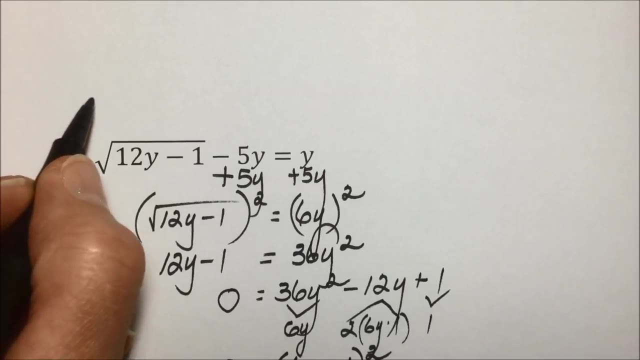 one sixth, Is it a solution to tell that We would plug it back in and test to see if it gives us a correct or true answer, And I'm going to do my check above the problem so that we can see what the original problem was? We're going to take 12 times y, which is one-sixth. 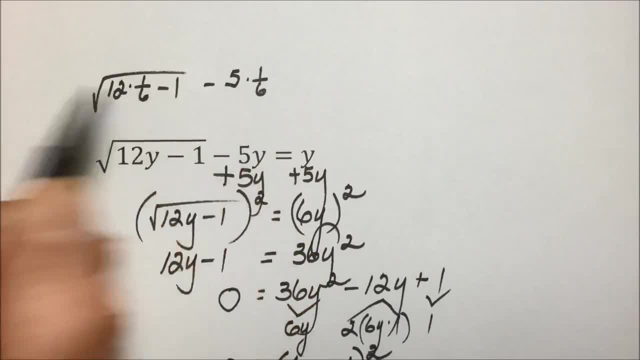 minus 5, times 1, 6th, and see if it equals 1- 6th. Well, 12 times 1, 6th is 12, 6.. 12: 6 reduces to a 2.. 2 minus 1 is 1.. The square root of 1 is 1.. 1 minus 5, 6.. To subtract those, we need a. 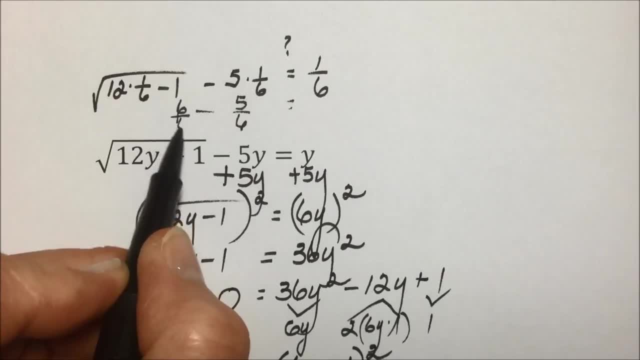 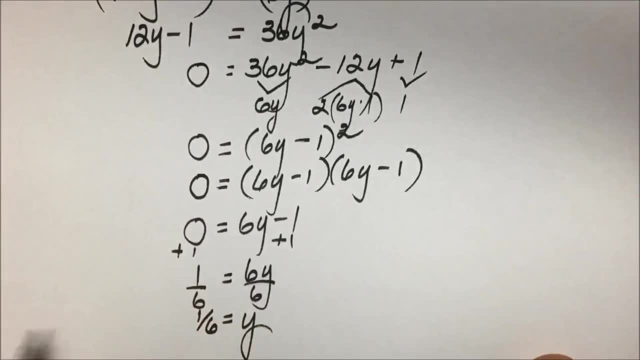 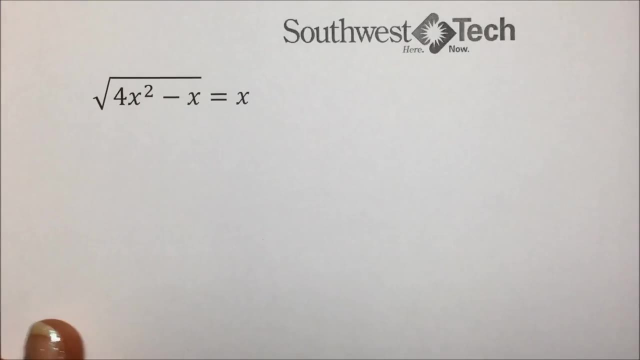 common denominator 1 is equivalent to 6, 6.. 6, 6 minus 5- 6 leaves us with 1- 6th. Our solution is correct. Here we have another radical equation. The radical is by itself. We are going to next. 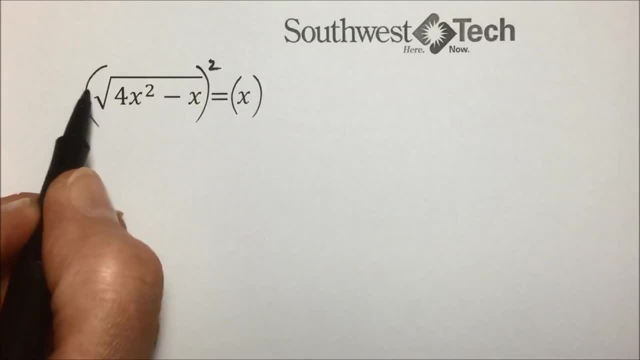 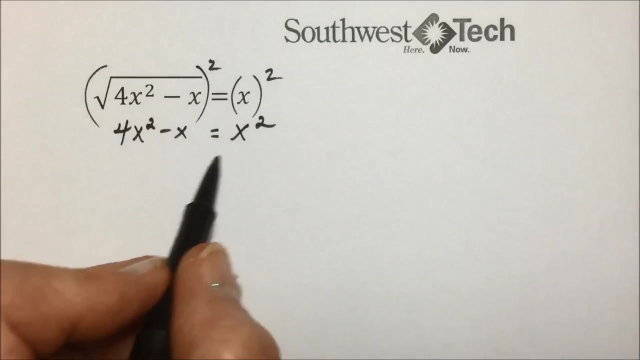 use our principle of powers To undo a square root. we will raise each side of the equation by 2. Squaring a radical gives us the radicand of 4x squared minus x is equal to x squared. Getting our like term. 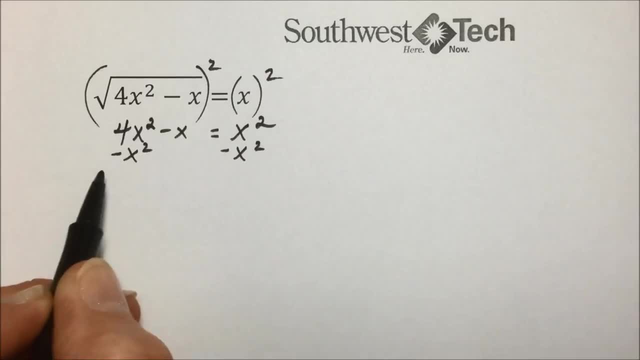 terms together. subtract an x squared from each side leaves a 3x squared minus x is equal to 0.. We're left with factoring. We have two terms and we're looking for a greatest common factor. We have an x common to both. That leaves a 3x minus 1.. We have a product. 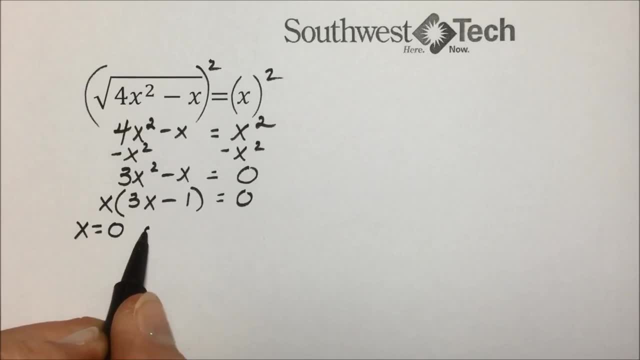 equal to 0. That means either the x is equal to 0 or 3x minus 1 equals 0.. Solving for x on this one. since we already have this solved, we'll add a 1 to both sides. That leaves a. 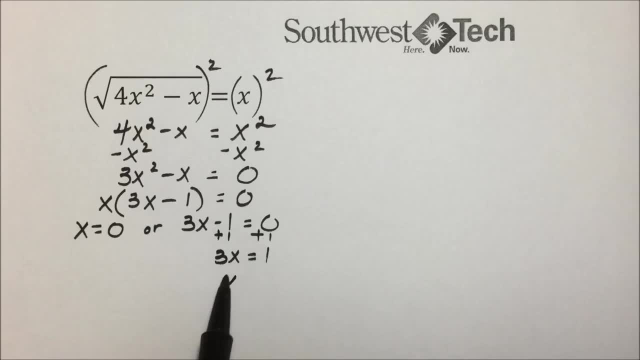 3x is equal to 1. And divide both sides by 3. We end up with x is equal to 1 third. So it's a possibility that we have two solutions, And let's see if these values are true. Let's see how these work If we plug in a 0 in our original equation, 4 times 0 squared. 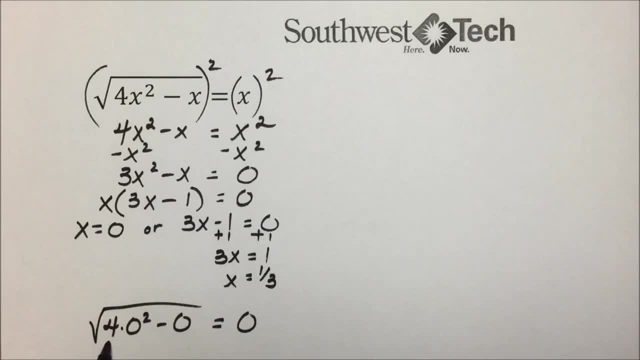 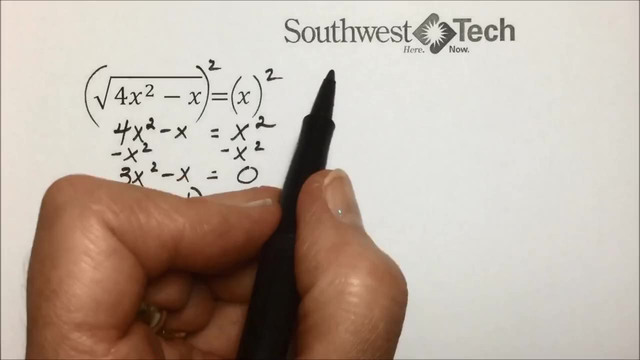 minus 0, does it equal 0 when we take the square root of it? Well, 0 squared is 0 times 4 is 0.. 0 minus 0 is 0.. Square root of 0 is 0. It works. 0 works. Does 1 third work? Well, 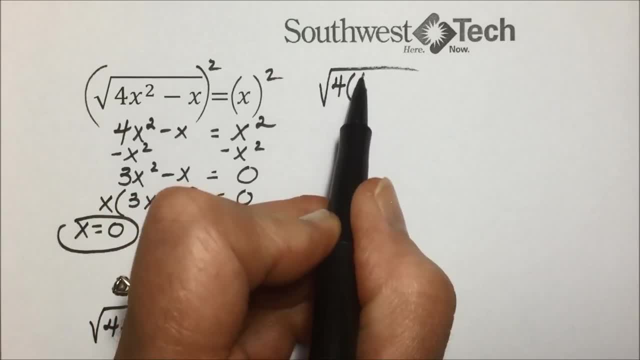 let's check it out 4 times. 1 third square root of 0 is 0.. Does 1 third square root of 0 work? Does 1 third square root of 0 work? Does 1 third square root of 0 work? Does 1? 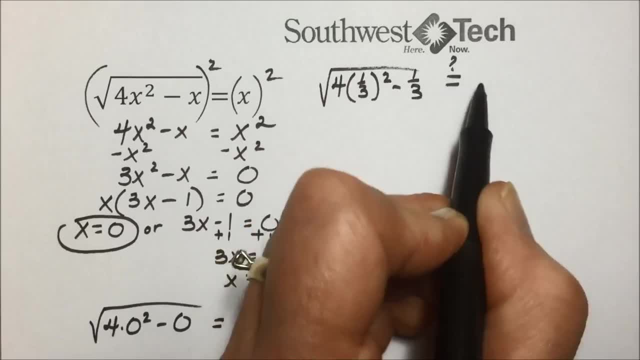 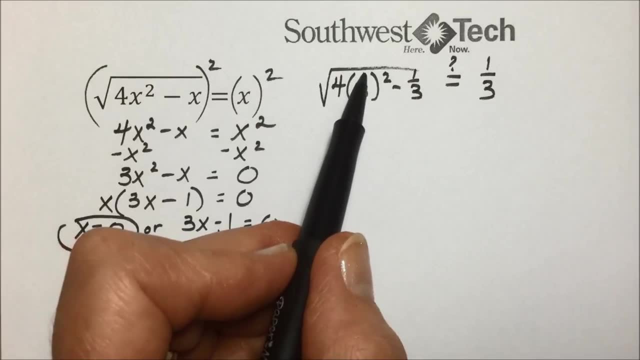 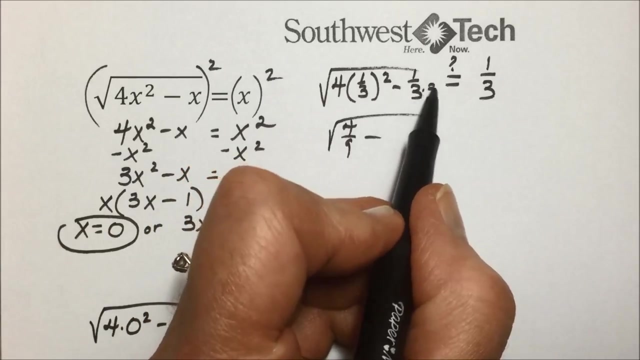 squared minus one-third. Does it equal one-third? if we replace x in our original equation Following order of operations, one-third squared is one-ninth times four is four-ninths. We have four-ninths minus one-third. One-third, if I multiply top and bottom by three, is 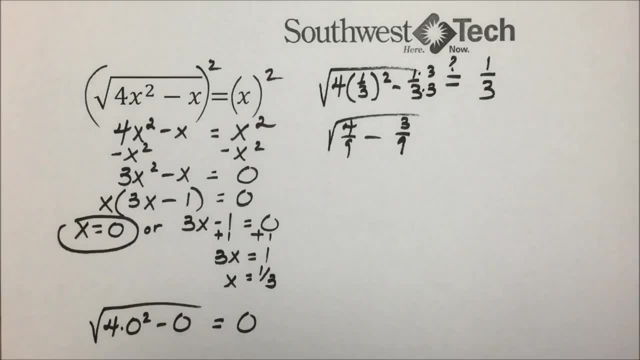 three-ninths, and taking four-ninths minus one-ninth leaves us with- I didn't say that right. four-ninths minus three-ninths leaves us with one-ninth. and taking the square root leaves us with one-third, which is equal to our solution. So that also is a solution. 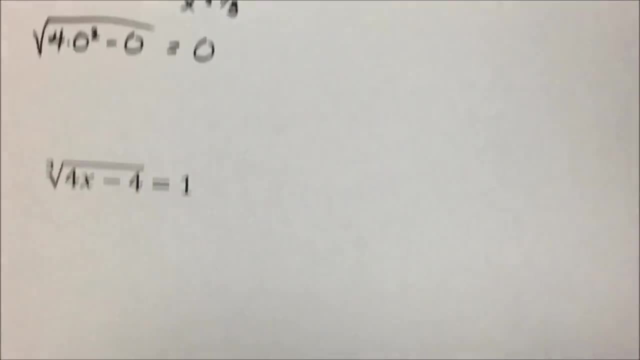 solution to this problem. In this last one we have a radical equation. Nothing says that the radical has to always be a square root. No problem. The principle of powers: as long as you raise both sides to the same power, we essentially maintain equality. Not always. 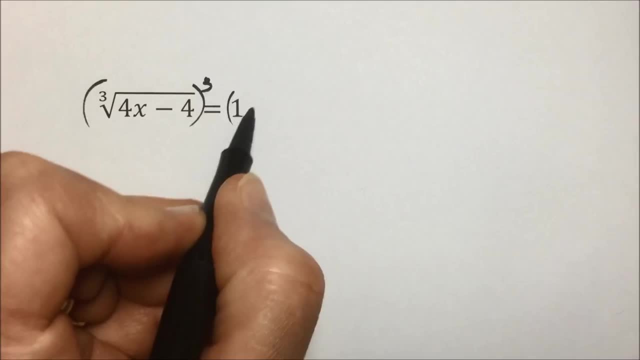 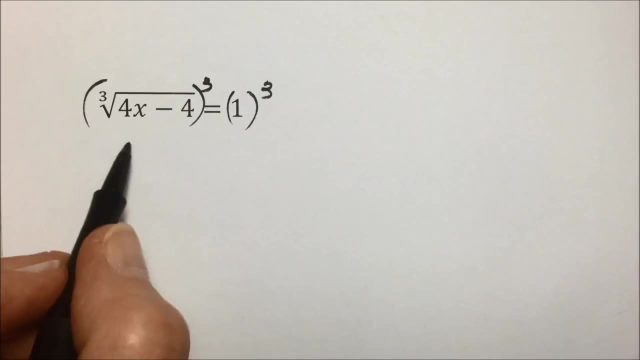 true and that's why we're checking our roots. So we're going to raise, in this case to undo a cube root. we'll raise each side to the third power. The cube root of three-ninths goes in one quarter, which is to the third power, or we're going to add a third power.